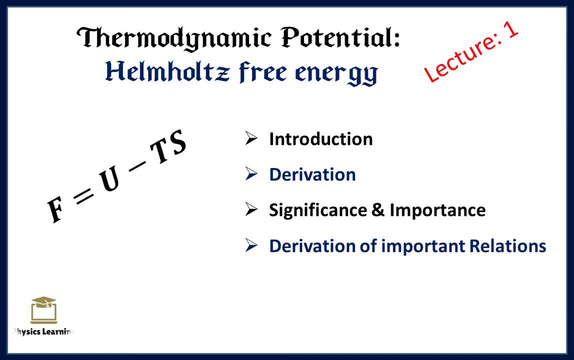 Welcome. in this video I am going to discuss about Helmholtz free energy. This is one of the thermodynamic potential, So in this video I am going to derive it, I am going to discuss about its significance and then, finally, we will going to see some of the important relation derived using Helmholtz free energy. So let's start. 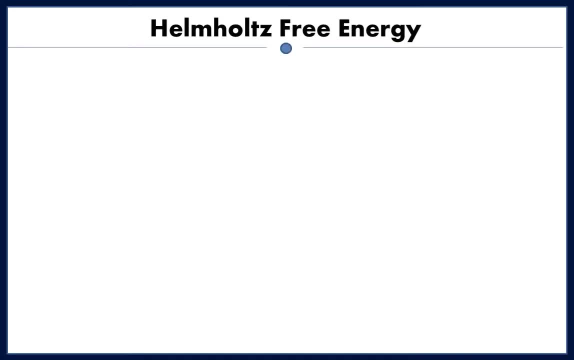 Helmholtz free energy. So how the concept of Helmholtz free energy came In classical mechanics. what we know, that amount of work done by a system is equals to decrease in the energy of the system. We can write mathematically like this: Delta W. that means amount of work done is equals to decrease in the energy. This minus sign signifies the decrease. 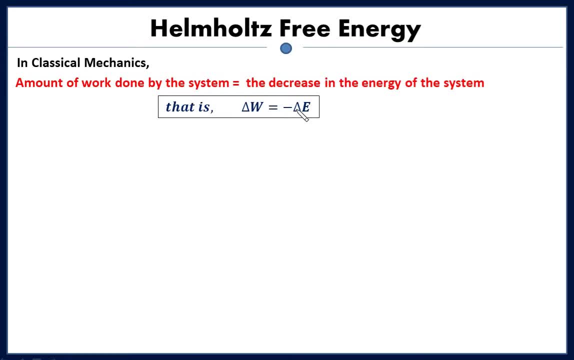 So this work done equals to decrease in energy. Do we have similar kind of relation in thermodynamics? To answer this question, let's review the thermodynamical system and we will use first law of thermodynamics here. Any thermodynamical system, or specifically I can say the state of any system in thermodynamics, is specified here. 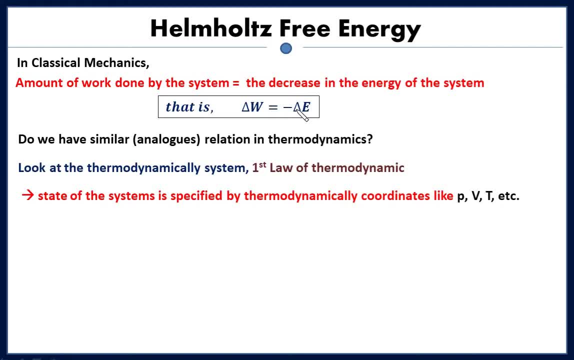 By thermodynamical coordinates. Like, suppose you have a gaseous system, then in order to define the state of system, what you can use is pressure, volume, temperature. So if I say that this gas have this much of pressure, this much of volume, this much of temperature, then in that way we can completely give the idea about that system. 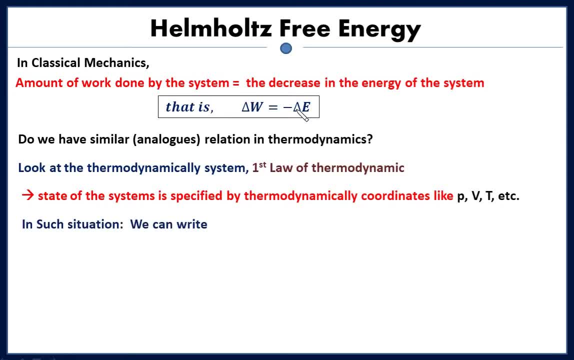 Okay, So in such scenario what we can write, that work done by that system that is delta W, is equals to change in internal energy plus heat absorbed by that system. What it means? that if you supply some amount of heat to that gaseous system, then it will absorb some heat and that heat will be utilized by that system in two ways. 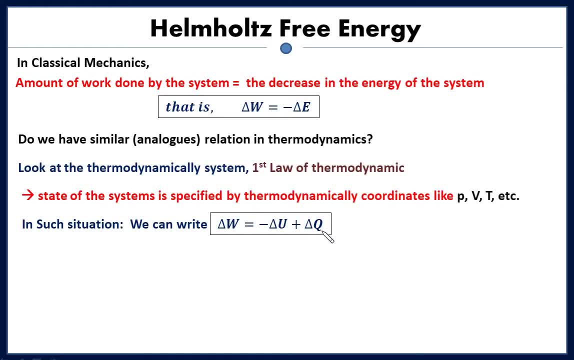 First it will change its own internal energy and then it will perform some amount of work. So this relation came from first law of thermodynamics, Which says that delta W equals to minus delta U plus delta Q. Okay, So here delta Q is a heat exchange between system and surrounding. 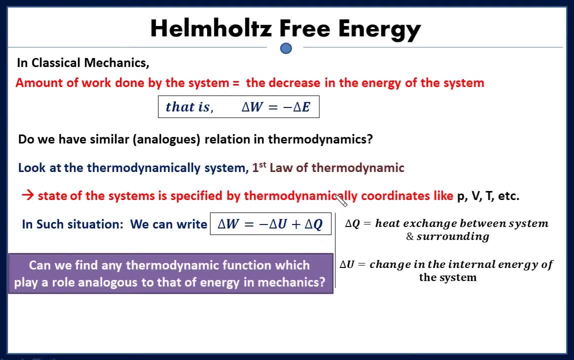 What we have seen here, that this two equation not look similar. So can we have that? So can we have some kind of function which play analogous role of this energy in classical system? In classical system we have energy. So in thermodynamics can we have something equivalent to this energy? 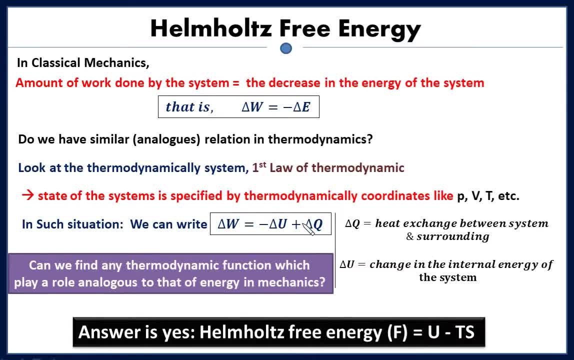 Answer is yes, we have. That is Helmholtz free energy, which is given by a symbol, F, and which is written as means which is equals to U, Internal energy of the system minus T S. Here T is the temperature of that system and S is the entropy of that system. 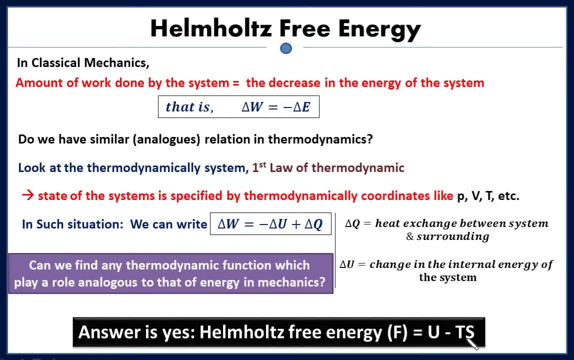 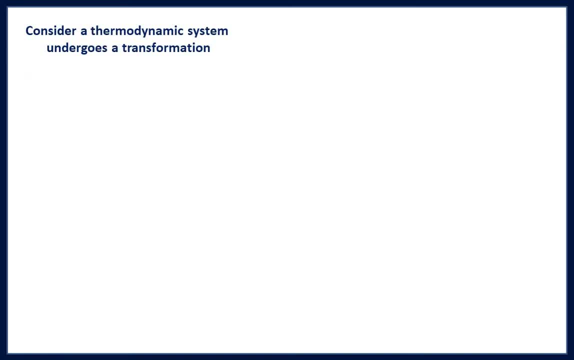 So F equals to U minus T S. So that's how the concept of this Helmholtz free energy came. Let's derive this expression. So consider a thermodynamical system undergoes a transformation. Suppose we call this as a initial state. 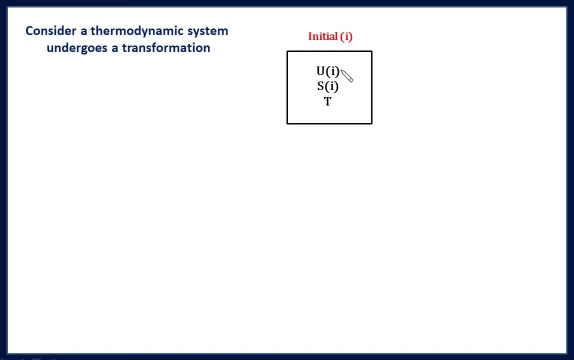 And this state is defined by Internal energy U, Entropy I and temperature T. This undergoes a transformation. We assume isothermal transformation, Which means the temperature will be constant throughout transformation And initial and final state must have same temperature. Let's say the final state has entropy. 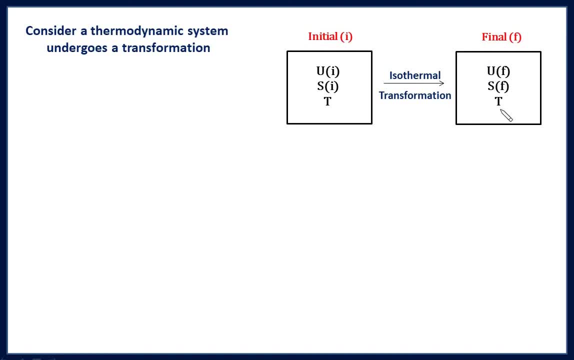 Sf, Internal energy, Uf and temperature T. And under this transformation, Delta W is the amount of work done by the system And heat exchange is delta Q. So this is complete setup for this transformation. Now from the Clausius theorem, what we know is this: 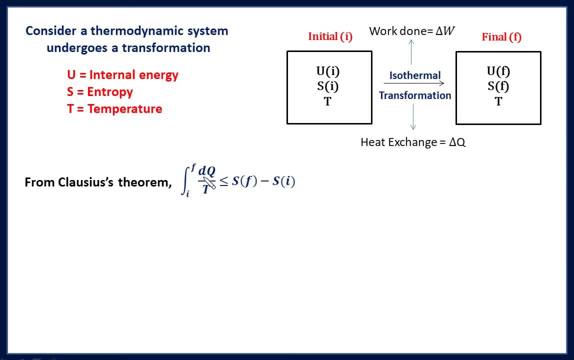 Here dQ is amount of heat exchange in infinitely small transformation. Like if you are going from I initial state to final state, Then you just divide this transformation in very smaller steps. So this dQ is that amount of exchange in that infinitely step during this transformation. 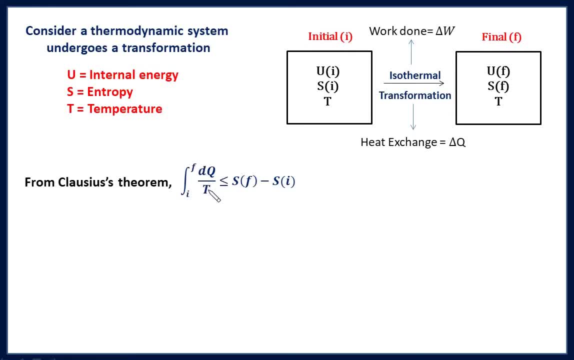 So if you divide this dQ by T And if you sum over all these steps, That is, integrate over I to F, This factor will be either less or equals to change in the entropy of the system. So if Sf is the final, 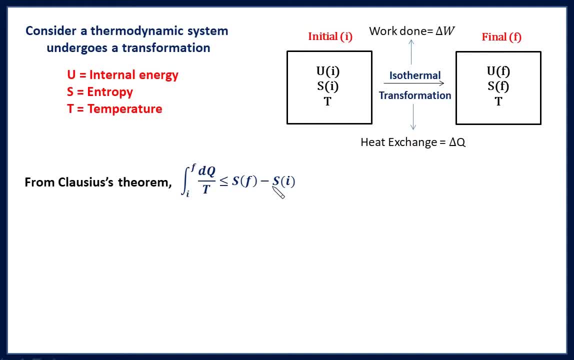 Entropy And Si is the initial entropy, Then this factor must be equals to Sf minus Si. Here equals to valid for the reversible transformation And less than is for the irreversible transformation. Let me explain what is reversible transformation. Reversible transformation, that suppose you goes from initial state to some final state, F. 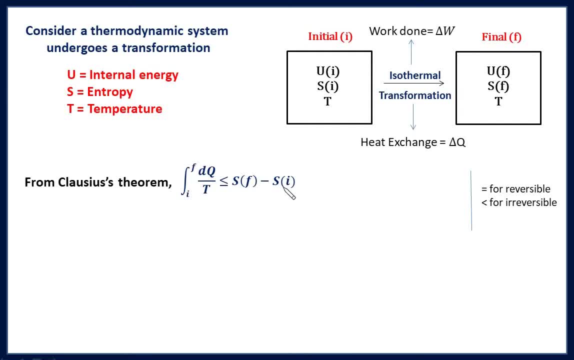 By somehow, if you can bring back the system F to I Without changing anything, Like if you come back to I, Everything will be exactly similar to the previous case. In that scenario we say it is a reversible And otherwise it is irreversible. 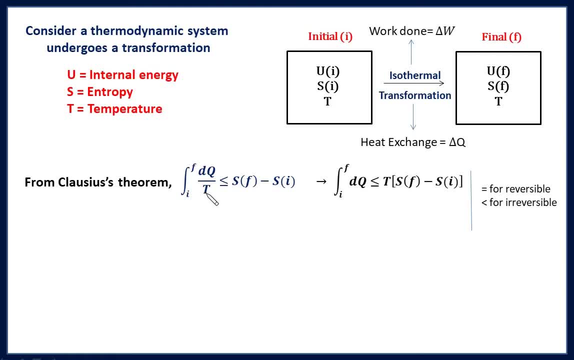 Now T is constant, So we can simply take it out from the integration. We multiply this side. If you perform this integration, It must be total heat exchange from initial to final state, So we can write as delta Q, As we assume that heat exchange is delta Q. 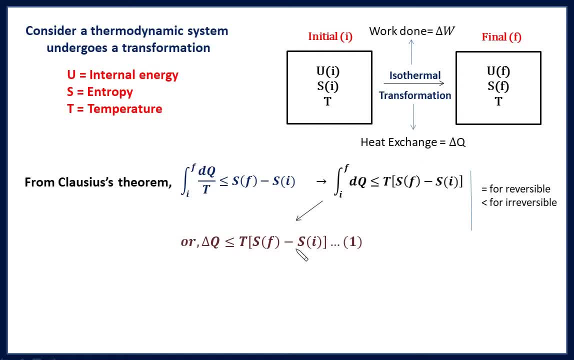 So delta Q is less than equals to T into Sf minus Si From first law of thermodynamics. As I have discussed a while ago, That delta Q heat absorbed by the system will be utilized in two way. First, it will change the internal energy of the system. 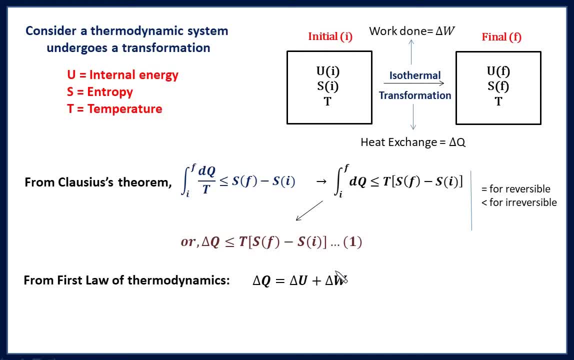 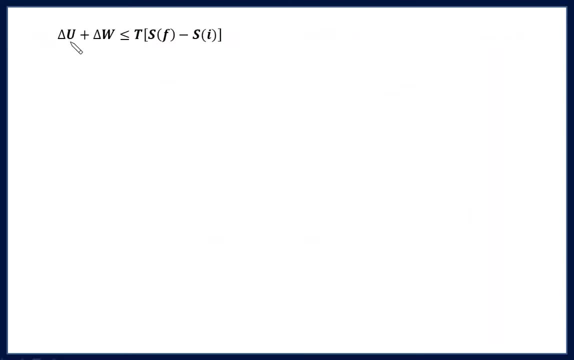 Plus amount of work done by that system. So if we combine these two, We can write: delta U plus delta W- is less than equals to T- into Sf minus Si. Now what is delta U? Delta U is change in internal energy. That means Uf minus Ui. 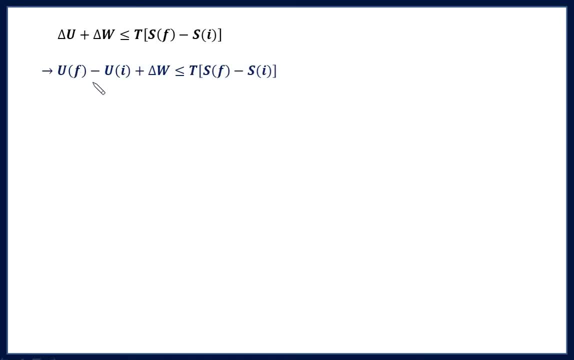 So just substitute that Uf minus Ui plus delta W is less than equals to T into Sf minus Si. Let's rearrange it So we can write: delta W is less than equals to Ui minus TSi. We have brought these two terms in the right hand corner. 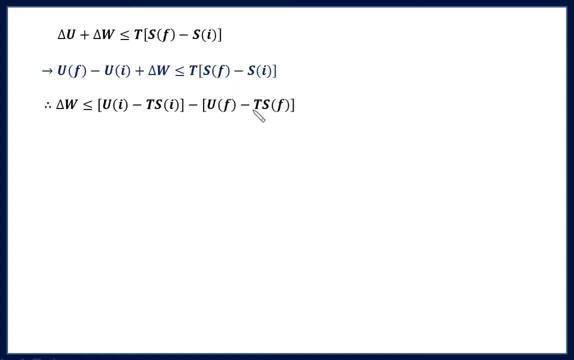 In the right hand side: Minus Uf, minus Tsf. Let's introduce one function, F, which is equals to U minus Ts. This is nothing but Helmholtz free energy. So from this, If we substitute Ui and Si, 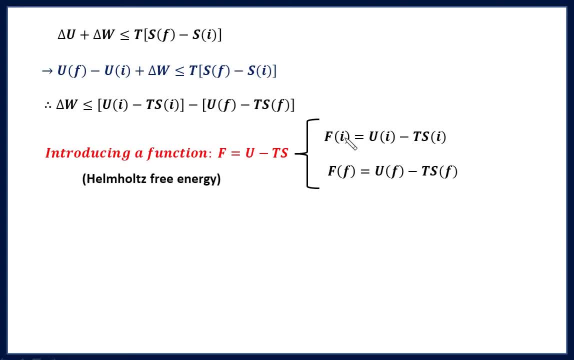 Then this is nothing but Fi. That means Helmholtz free energy in the initial state. Similarly, Helmholtz free energy in the final state can be written as Uf minus Tsf, As T is the same for initial and final state. 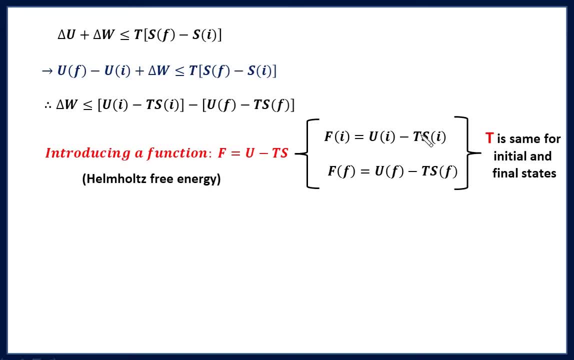 So we are not using any kind of I or F to defining the temperature. Thus the final relation become: delta W is less than Fi minus Ff, Which is equals to minus delta F. Delta F is change in Helmholtz free energy. 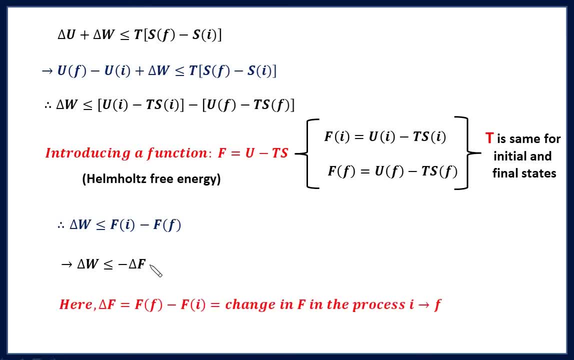 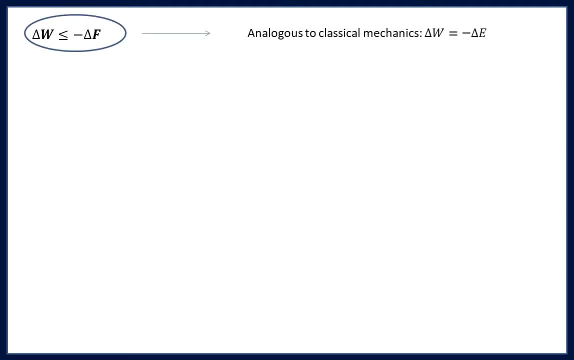 Which is Ff minus Fi. Now look at this. So this looks exactly analogous to classical mechanics Where delta W is equals to minus delta E. Here it have less than equal to, Because we have considered two process, irreversible and reversible. So what we can say from this relation? 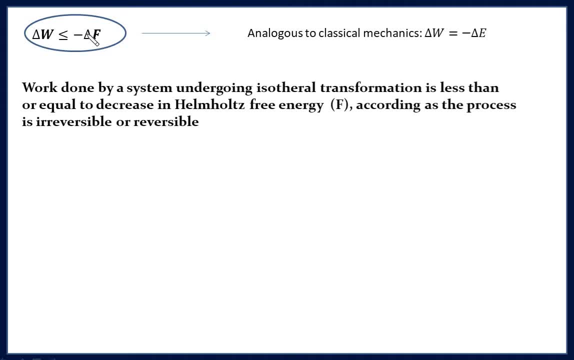 Work done by a system undergoing isothermal transformation Is less than or equals to decrease in the Helmholtz free energy And equals to for the reversible case and less than for the irreversible case. So if you consider only the reversible transformation, Then Helmholtz free energy playing exact role of energy. 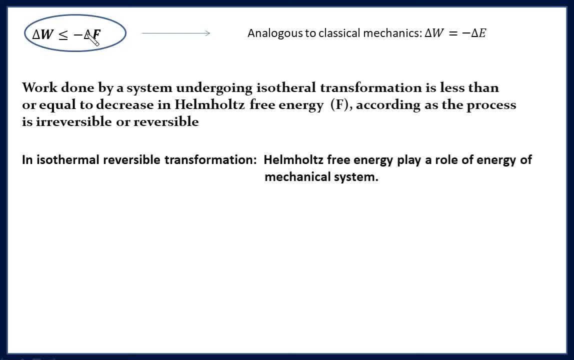 Of classical mechanical system. So if somebody will ask you to just define Helmholtz free energy, Then you can just start with writing this expression That Helmholtz free energy is given by internal energy minus temperature into entropy, And it signifies by this work done. 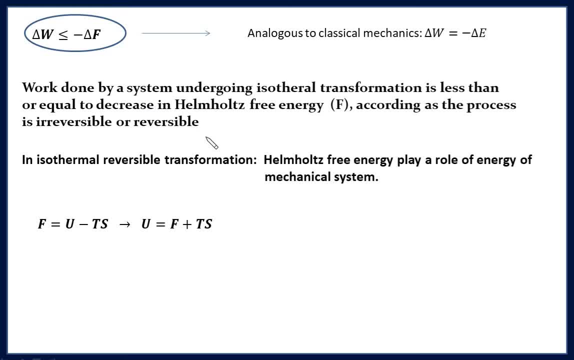 And then you can write this statement and so on. So let's try to have some deep insight in it. So in Helmholtz, free energy F is equals to U minus TS. So if you rearrange this, Then U, which is internal energy of a system, is equals to F plus TS. 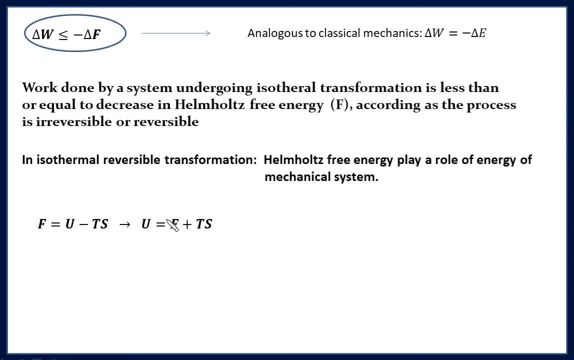 That means internal energy is made up of two parts: F, which is free energy, And TS, which we called bound energy. So this F, free energy is available for the work done And this bound energy is unavailable for the useful work. So suppose your system have some amount of internal energy. 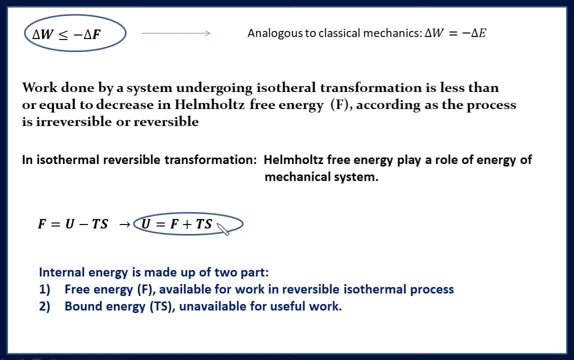 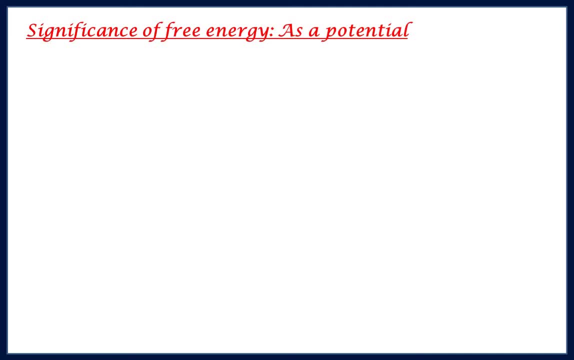 That means this energy can be utilized partially for the work done, And partially energy cannot be used for the work done. Now, as I started with the point that Helmholtz free energy is a thermodynamics potential, Let's see how we can understand this point. 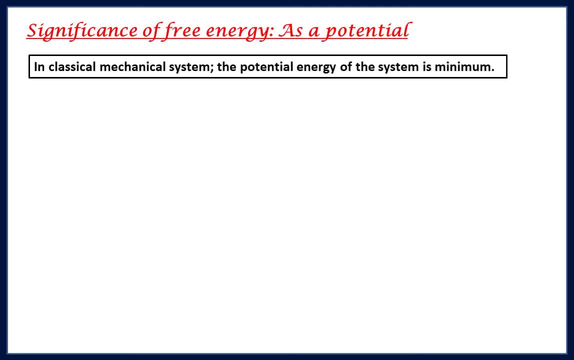 So in classical mechanics what we know, that potential energy of a system is minimum. So if you have any classical system, then your system try to be in a state which have minimum potential energy. Now we try to look same thing in the thermodynamical system. 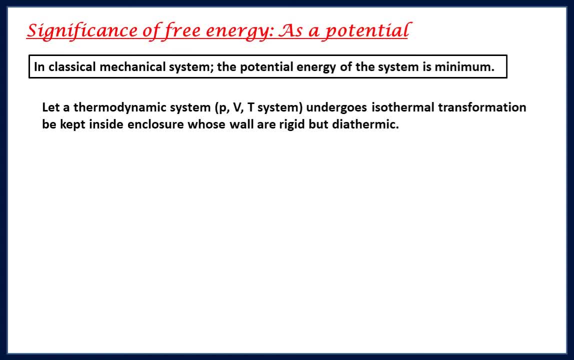 Let's assume a thermodynamical system like gaseous system. So we have PVT system, we call it, And this system undergoes a isothermal transformation. As we have seen, we have derived this free energy for the isothermal transformation And it is kept inside an enclosure. 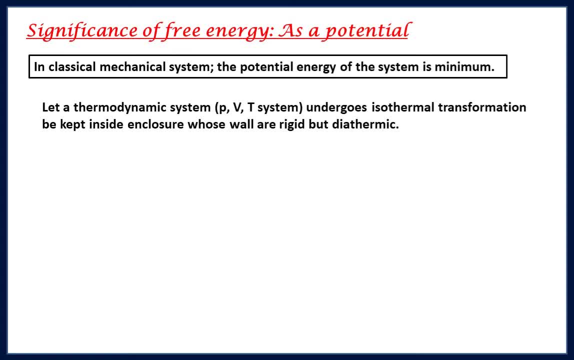 So you can assume any kind of box Whose walls are rigid, Means the wall cannot move, But diathermic, Which means it can exchange heat. So like this: And it has some piston, but piston is not moving, So this gas is trapped inside. 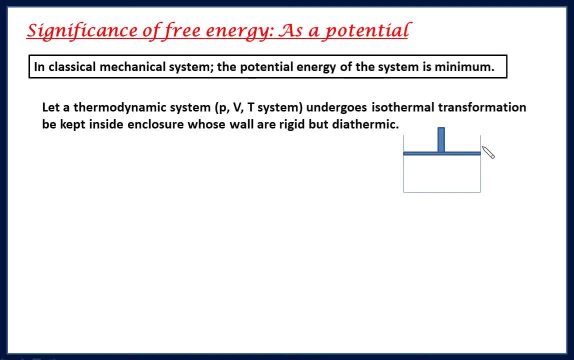 So wall can exchange heat with the outside, but nothing is moving. So if nothing will move, then the volume of the gas is constant, Right. So in PVT system the work done is equals to pressure into change in volume, But as volume will not change here because this is rigid. 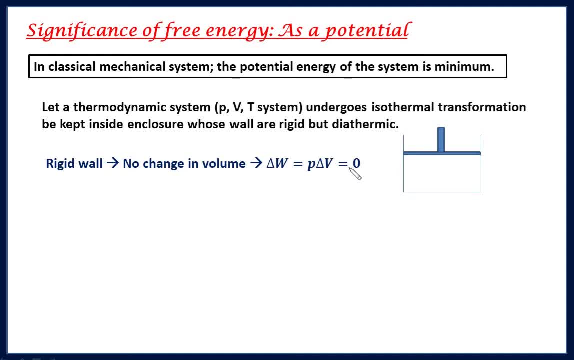 So work done equals to zero. Thus we know that delta W is less than equals to minus delta F. So now this delta W is zero because there is no work done in such scenario. So if you substitute delta F, which is FF minus Fi, 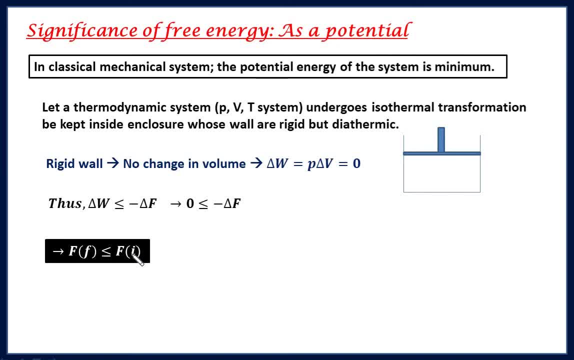 What we can see. FF is less than equals to Fi. The Helmholtz free energy in the final state is always less than equals to Helmholtz free energy in the initial state, Which means free energy. Helmholtz free energy in final state can never exceed that in the initial state. 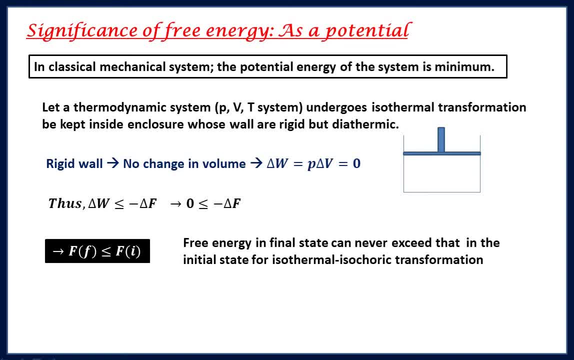 For isothermal and isochoric transformation. Okay. Isothermal means there is no change in temperature. Isochoric means no change in the volume. Your system try to be always in that stage where the this Helmholtz free energy is lower. 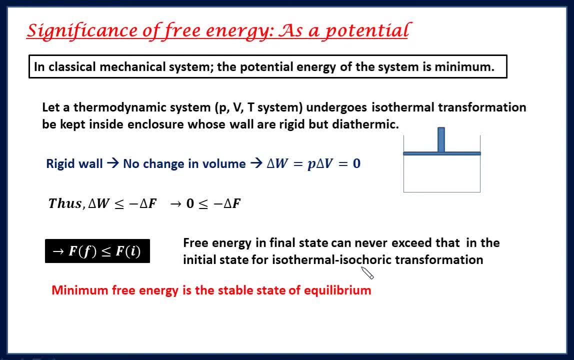 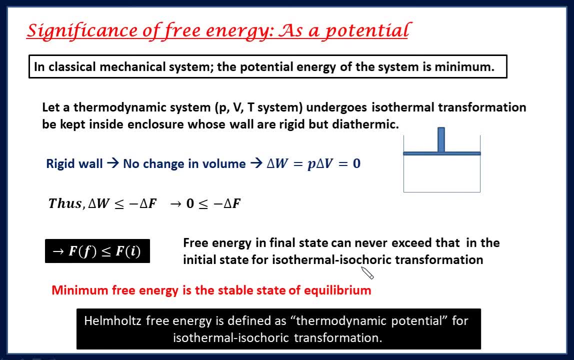 So the minimum free energy means stable state of equilibrium. Thus this Helmholtz free energy is a thermodynamics potential for a particular case of transformation where temperature and the volume is constant. Okay, So if you have any system and it going under some transformation, keeping is temperature and volume constant. 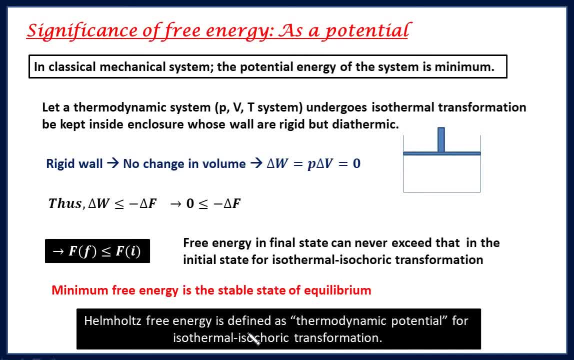 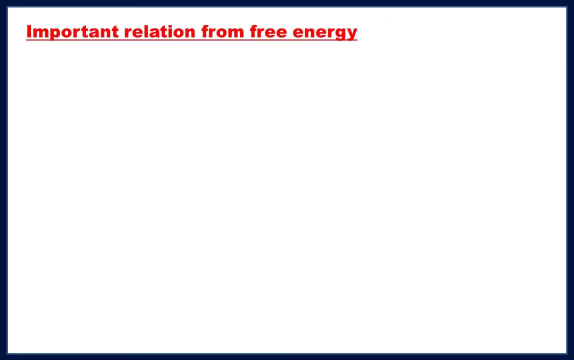 Then, in that kind of transformation, This Helmholtz free energy playing a role similar to the potential. That's why we call it a thermodynamic potential. Now let's move to our final state, where we are going to derive some of the important relation from this Helmholtz free energy. 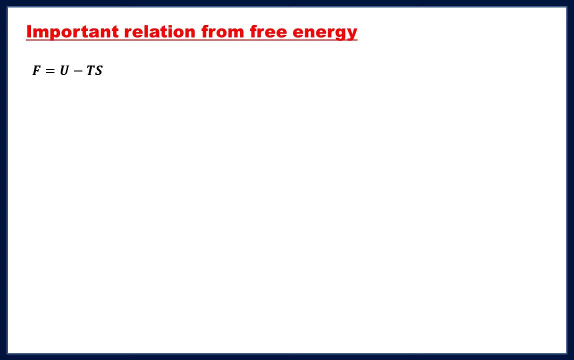 So this F is equals to U minus TS. We know that U, T and S are state variables. Okay, Means to define any system. you can also define U, T and S. These are the quantity which related to the particular state, So these are called state variable. 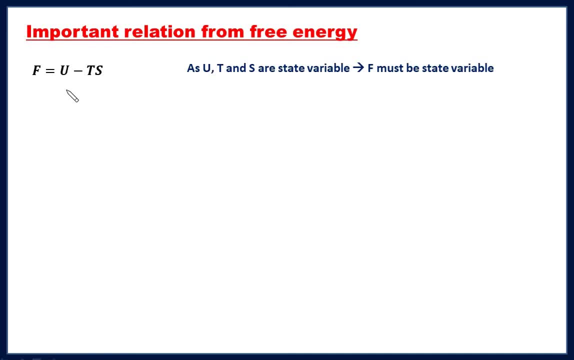 And as F is the combination of these, then F must be a state variable. Okay, Now suppose your system undergoes a very infinitely small transformation. Then if I'll ask you How much is the change in Helmholtz free energy? Then you can write. 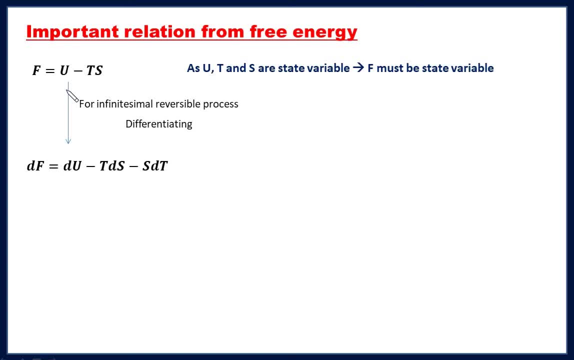 You can simply write, just by differentiating it. So DF equals to DU minus TDS, minus SDT. Let's look at one point From first law of thermodynamics: DQ equals to DU plus PDV. PDV is the work done. 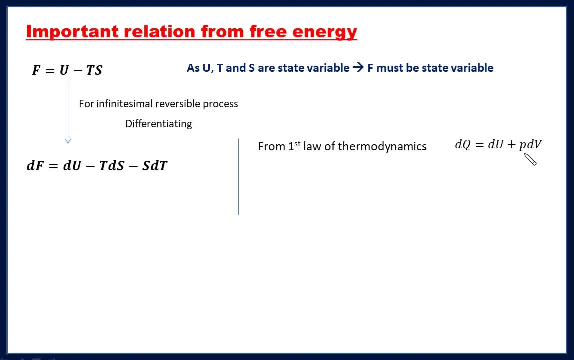 So DW is nothing but PDV For the PBT system. And from the second law of thermodynamics We know that TDS equals to DQ. So if you combine these two laws We can write: TDS equals to DU plus PDV. 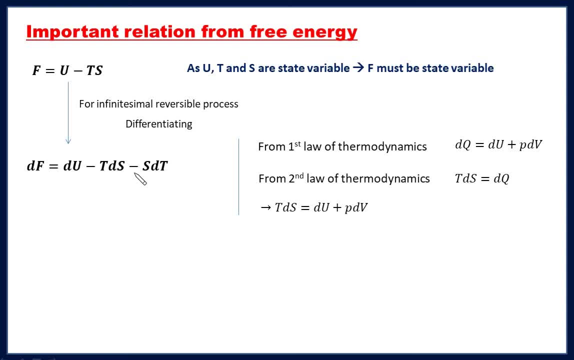 So we utilize this And we substitute here We can get DF equals to minus PDV, minus SDT. Let's call it relation 1.. What we have seen from here? That F is a dependent variable Which depend upon change in volume and change in temperature. 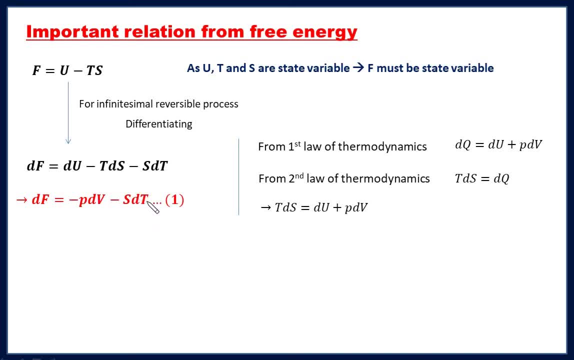 Which means V and T is the independent variable. These two variable we can tune independently from the outside. So F is dependent variable and V and T is the independent variable. So we can simply write F as a function of temperature and volume. So from this relation, 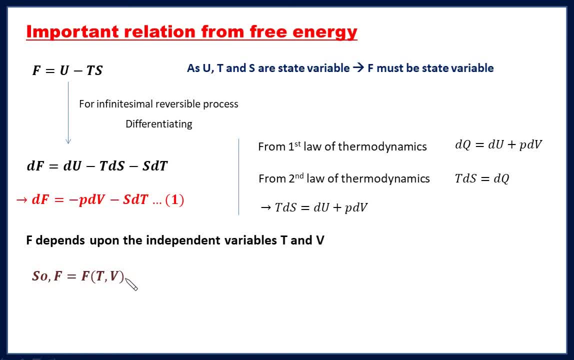 We can also find this change in F. So change in F is: DF equals to rate of change of free energy with temperature at constant volume into DT, Plus rate of change of free energy with respect to volume at constant temperature into DV. Ok, We can write this to this. 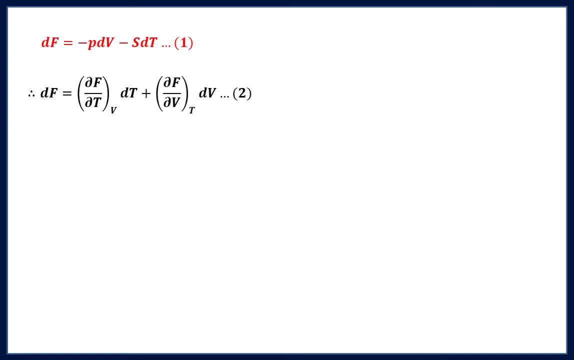 So now we have two different equation Which gives the value of DF, So we can simply equate it. And if you equate it or compare it, What you will find? That P equals to minus del F, del V at constant temperature. 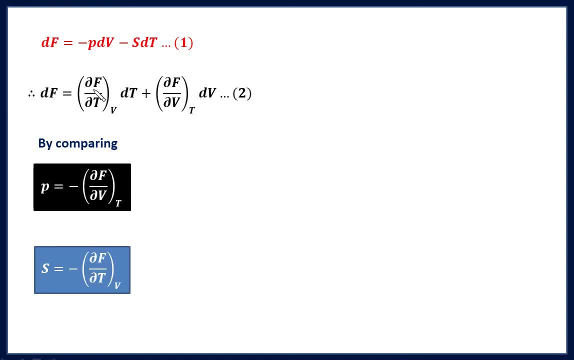 Similarly you can write entropy: It equals to minus del F del T at constant volume. So if you know this free energy, You can easily calculate the other parameters like pressure and entropy. So you can get complete information about the thermal property. Ok, 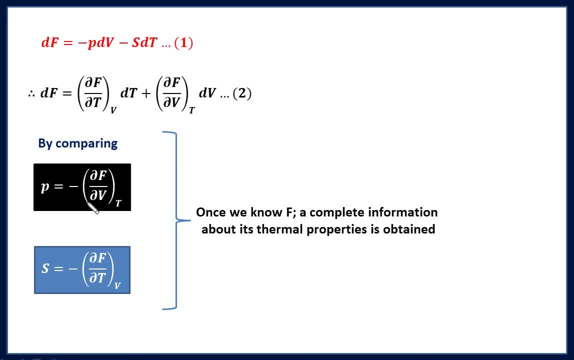 And what this first relation says- That if volume increases, Then free energy decreases. What the second statement says: If temperature increases, Free energy decreases. Ok, So hope these derivations and this all formula are clear to you. So I am stopping here. See you, Thank you.